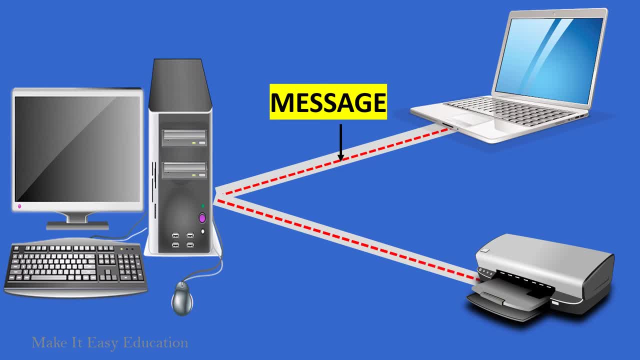 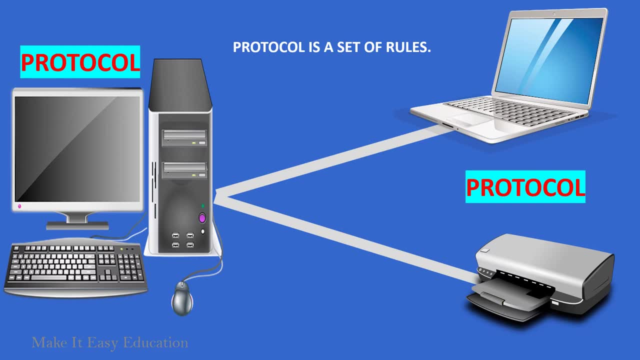 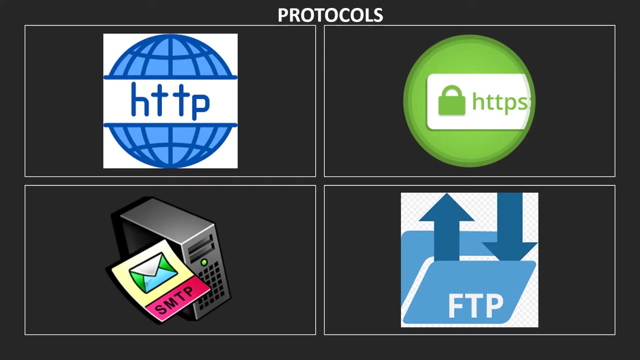 one device to another device over a computer network. A protocol is a set of rules that are agreed by both sender and receiver. Without a protocol, two devices cannot communicate with each other. For example, HTTP and HTTPS are the two protocols used by web browsers. 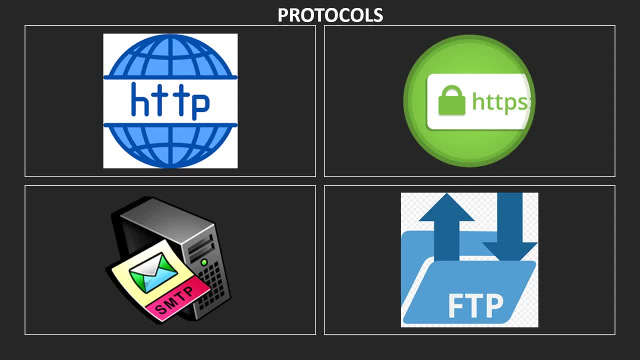 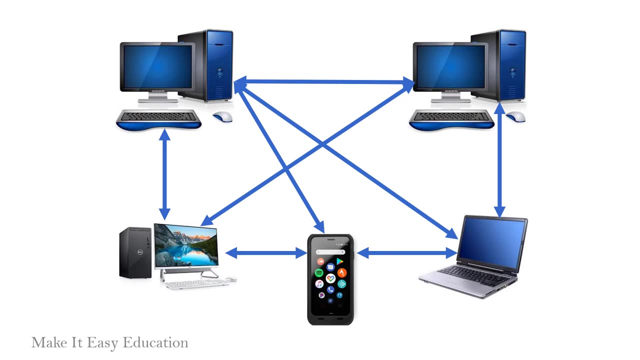 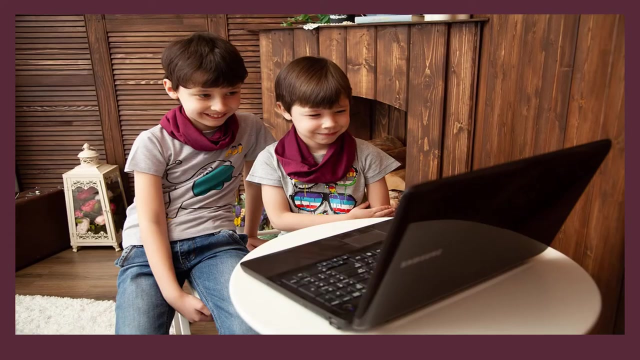 SMTP protocol is used by email services connected to the internet. The FTP is a standard network protocol used for the transfer of computer files on a computer network. Computer network transfer resources such as documents, pictures, videos, among devices Nowadays we use is computer network for entertainment. 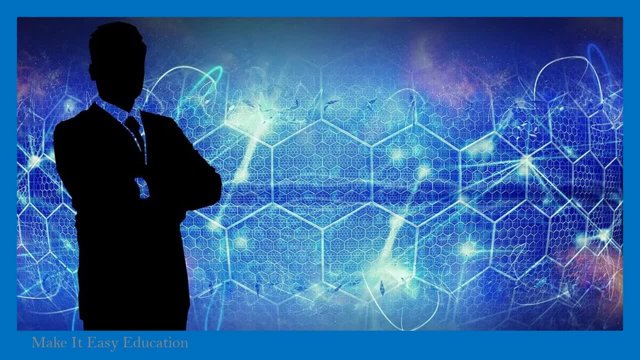 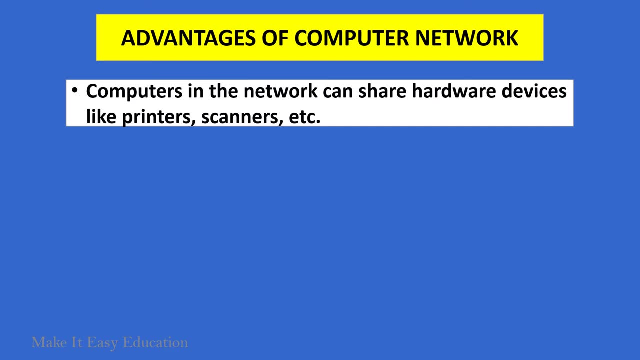 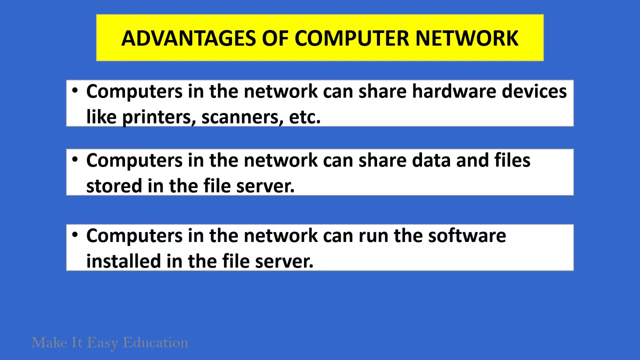 shopping and business Advantages of computer network. Computers in the network can share hardware devices like printers, scanners, etc. Computers can share data and files stored in the file server. Computers can run the software installed in the file server. Network users can exchange messages instantly. 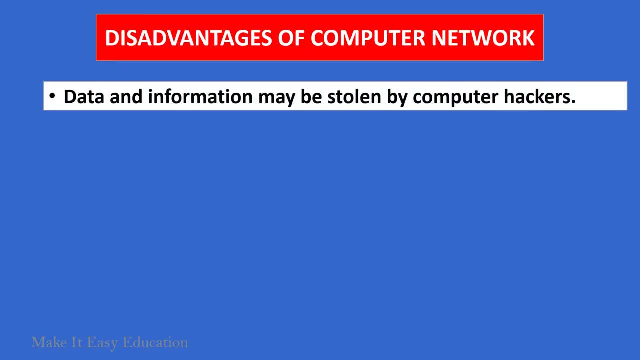 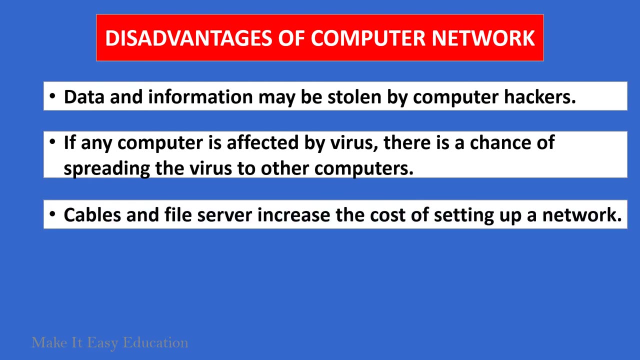 Disadvantages of computer network. Data and information may be stolen by computer hackers. If any computer in the network is affected by virus, there is a chance of spreading the virus to other computers. Cables and file server increase the cost of saving. 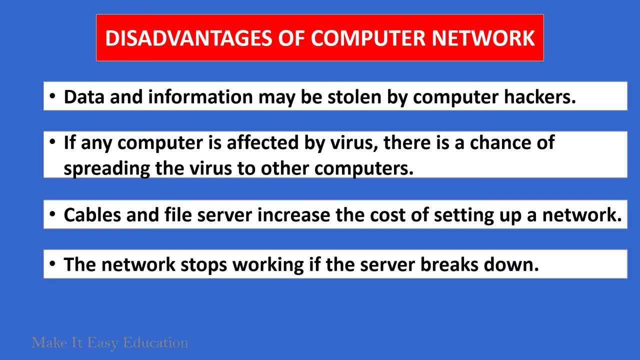 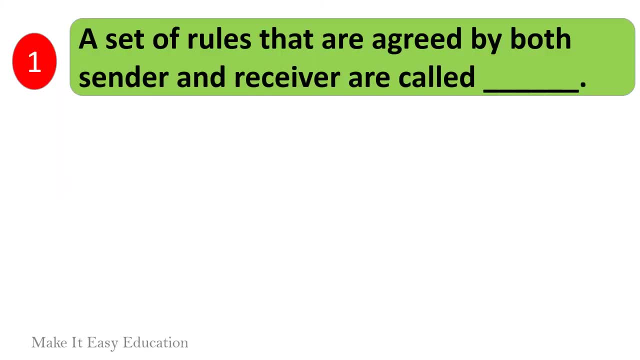 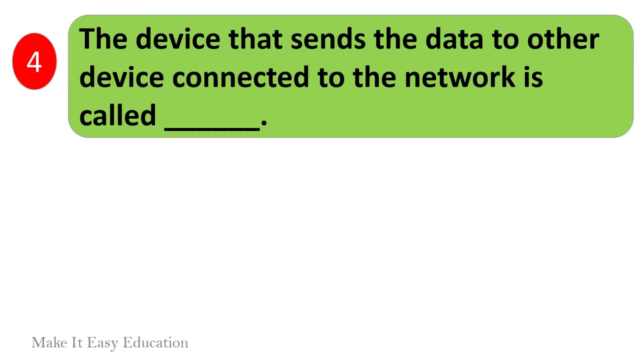 Cables and file server increase the cost of setting up a network. The network stops working if the server breaks down. Network manager and technicians are needed to run a large network. Question time Outline 2-2-1-1- management Identischer Test.